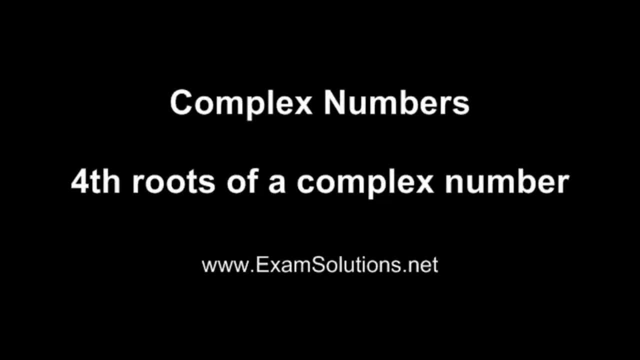 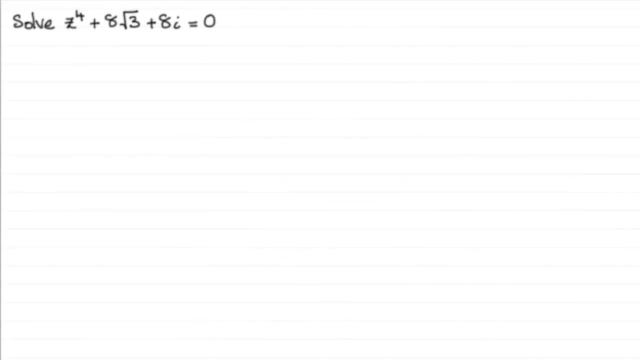 Hi. now this is another video in my series on finding the nth roots of a complex number, And we use DeMarva's theorem for these examples because it greatly simplifies the method of solution. So we've got here: solve z to the power. 4 plus 8 root. 3 plus 8i equals 0. 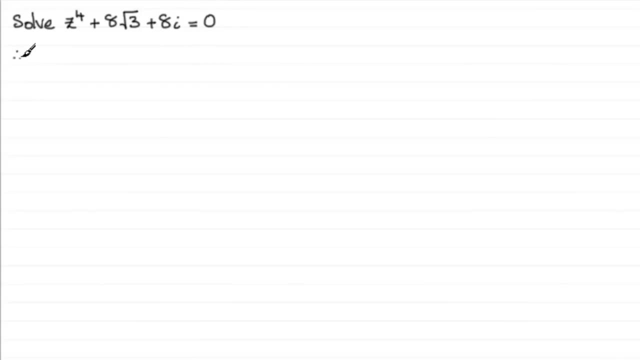 And if I was to rearrange this by subtracting 8 root 3 and minus 8i from both sides, it would give me that z to the power 4 equals minus 8 root 3 and then minus 8i. So to find z I'm going. 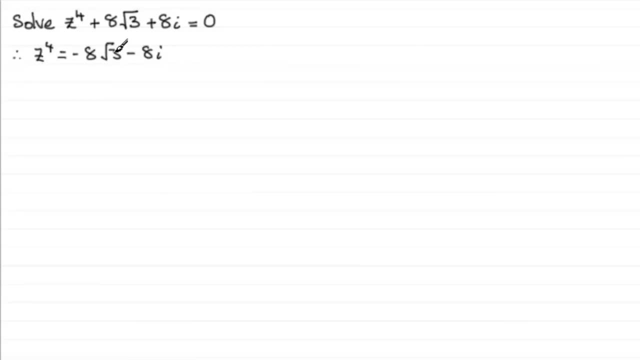 to need to find the nth root of a complex number. So I'm going to need to find the nth root of a complex number, So I'm going to need to take the fourth root then, of minus 8 root: 3 minus 8i. 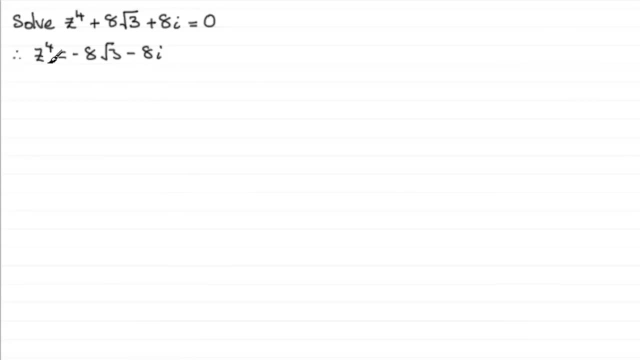 But before I do that, what I want to do is draw on an argon diagram- z to the power 4, work out the modulus and the arg of it, and then I can write z to the power 4 in modulus argument form. Now, to save time, what I've done is I've drawn up our argon diagram. 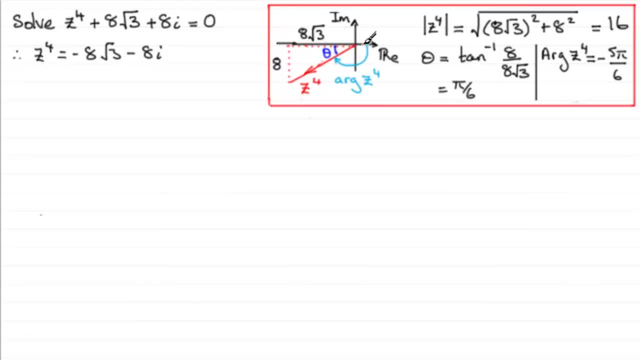 represented z to the power 4.. It's going to be minus 8, root 3 and minus 8i. So I've just taken off the negative signs here. All I'm interested in is the length of these two sides of this right angle triangle, So you can see that the modulus of z to the power 4 is going to be. 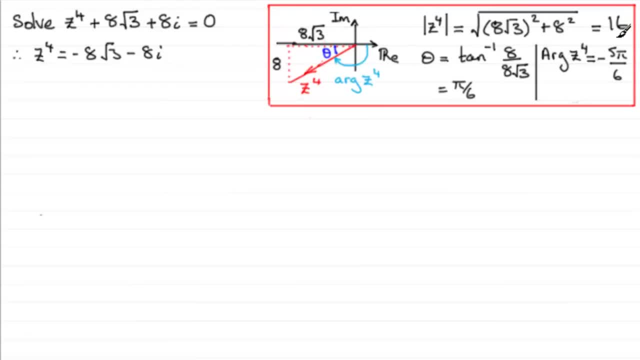 found by Pythagoras's theorem. It turns out to be equal to 16.. I've worked out theta in here, this acute angle. Theta is the inverse tan of 8 over 8, root 3, which turns out to be pi upon 6 radians. So therefore the arg of z to the power 4 has to be an angle. 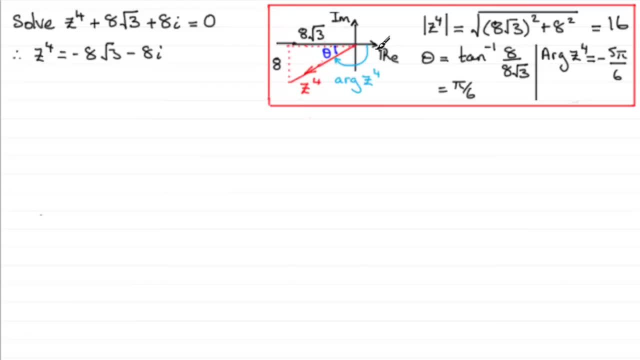 between minus pi remember, and pi radians. So I've had to turn in a clockwise direction. So arg of z to the power 4 is minus 5pi pi upon 6.. So I can now rewrite z to the power 4 in mod arg form. So its modulus then is going to be: 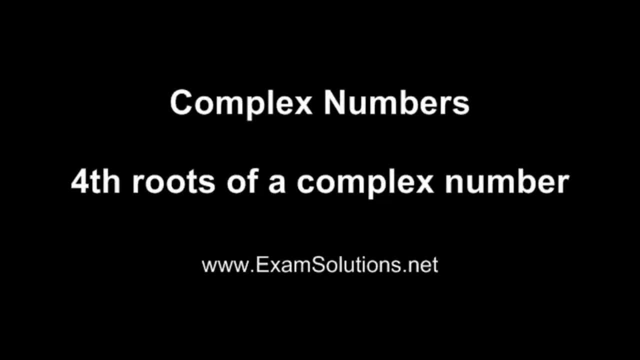 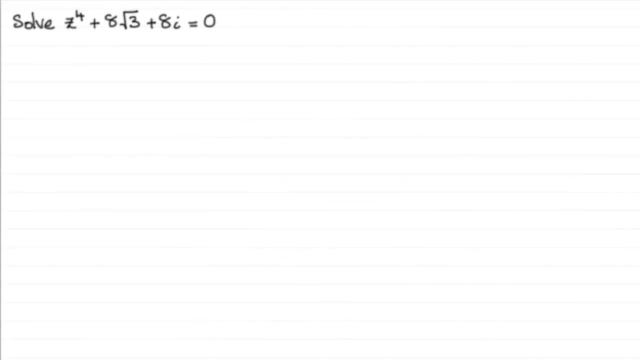 Hi. now this is another video in my series on finding the nth roots of a complex number, And we use DeMarva's theorem for these examples because it greatly simplifies the method of solution. So we've got here: solve z to the power. 4 plus 8 root. 3 plus 8i equals 0. 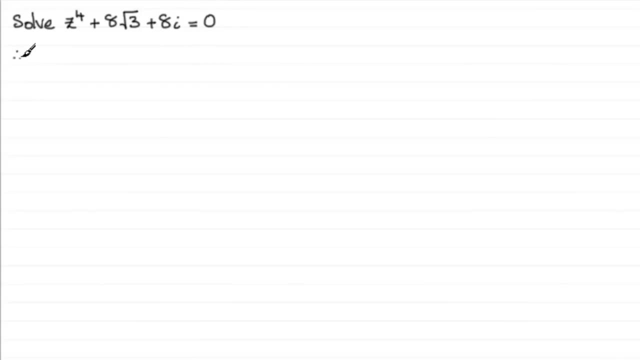 And if I was to rearrange this by subtracting 8 root 3 and minus 8i from both sides, it would give me that z to the power 4 equals minus 8 root 3 and then minus 8i. So to find z I'm going. 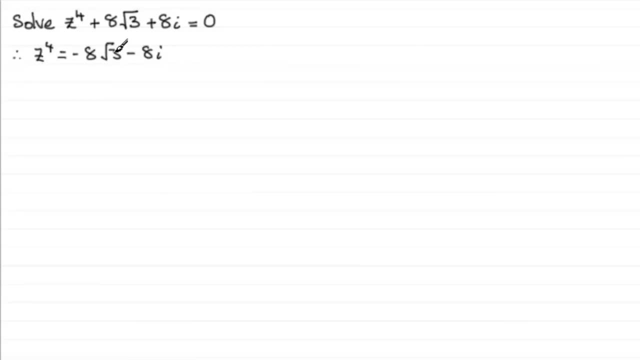 to need to find the nth root of a complex number. So I'm going to need to find the nth root of a complex number, So I'm going to need to take the fourth root then, of minus 8 root: 3 minus 8i. 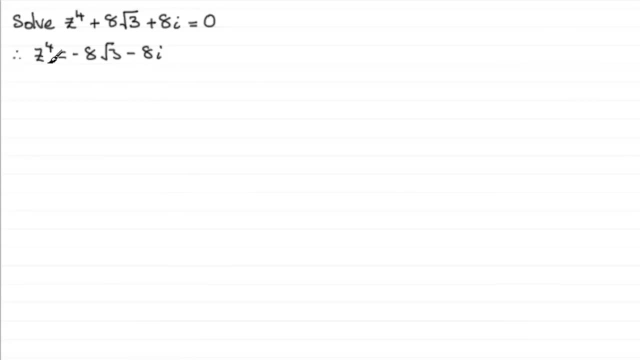 But before I do that, what I want to do is draw on an argon diagram- z to the power 4, work out the modulus and the arg of it, and then I can write z to the power 4 in modulus argument form. Now, to save time, what I've done is I've drawn up our argon diagram. 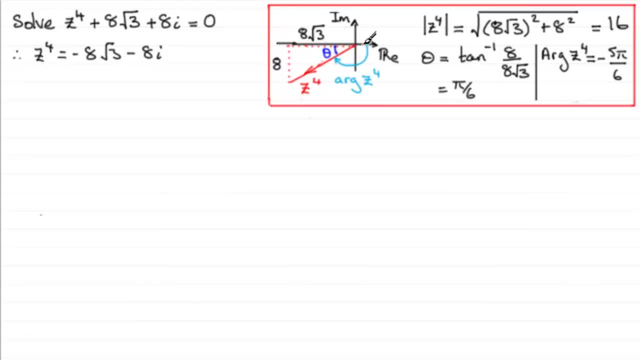 represented z to the power 4.. It's going to be minus 8, root 3 and minus 8i. So I've just taken off the negative signs here. All I'm interested in is the length of these two sides of this right angle triangle, So you can see that the modulus of z to the power 4 is going to be. 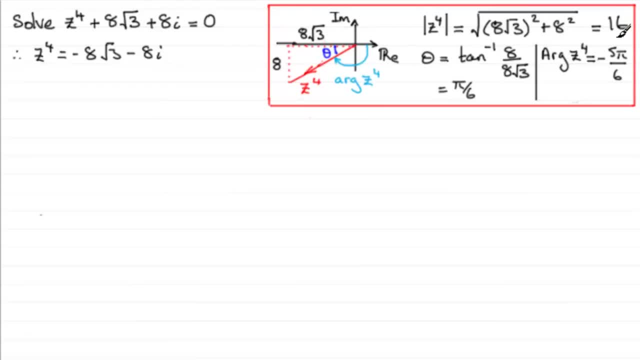 found by Pythagoras's theorem. It turns out to be equal to 16.. I've worked out theta in here, this acute angle. Theta is the inverse tan of 8 over 8, root 3, which turns out to be pi upon 6 radians. So therefore the arg of z to the 4 has to be: 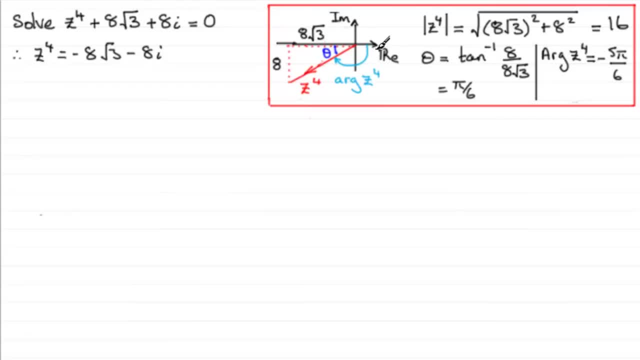 an angle between minus pi, remember- and pi radians, So I've had to turn in a clockwise direction. So arg of z to the power 4 is minus 5pi, So I can now rewrite z to the power 4 in mod-arg form. 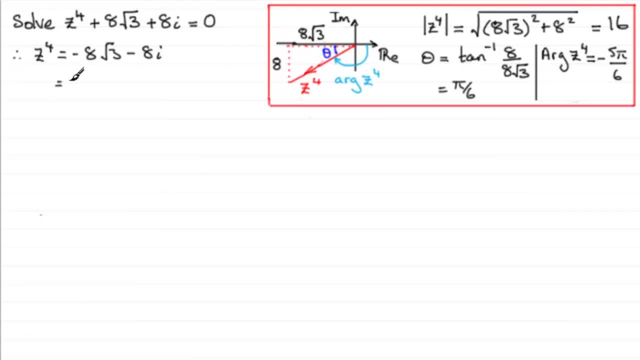 So its modulus then is going to be 16.. And then we can say that this is the same as the cosine of the arg, which is minus 5pi upon 6. So minus 5pi upon 6. And then plus 5pi upon 6.. 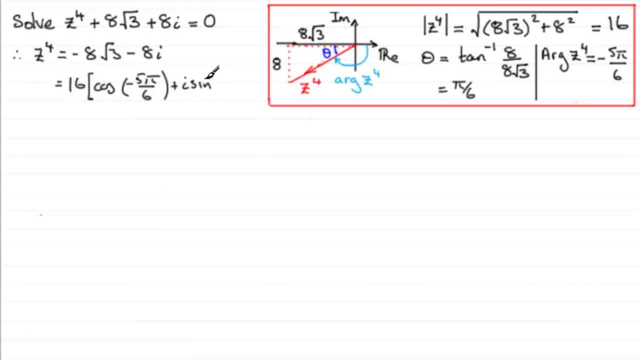 And then plus 5pi upon 6. I sine of minus 5pi upon 6.. Now this is going to have to be written fairly small, because we've got a lot to do in this small space, So I hope you'll understand that that it's going to feel a bit cramped. 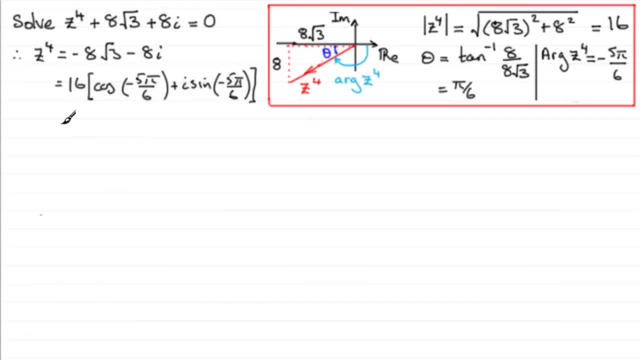 OK, well, what we now do, as I've shown you in the cube roots of 1, if you've seen that video- that we change this arg By adding 2kpi onto each of these angles here, Because we can turn in this direction. 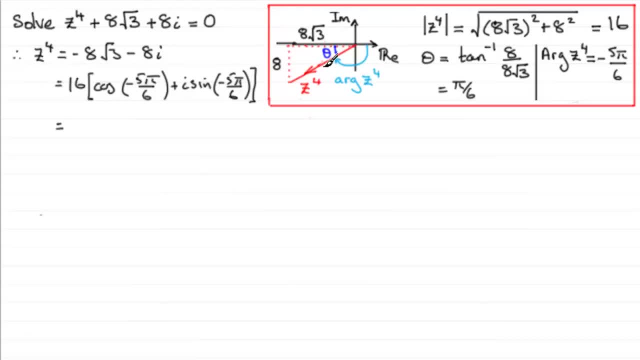 But if we add any multiple of 2pi onto this arg, It's always going to take us back to this position. So we'll just change this then to 16.. Multiplied by the cos of minus 5pi: So we'll just change this then to 16.. 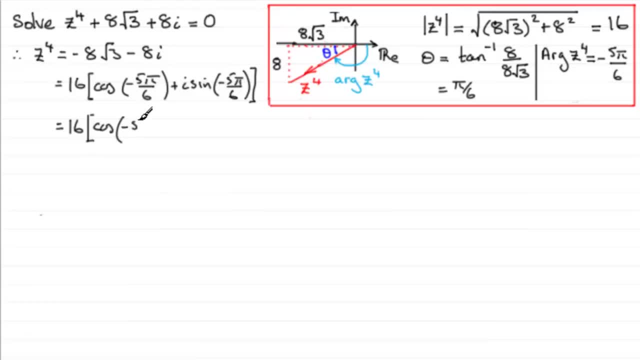 Multiplied by the cos of minus 5pi. So we'll just change this then to 16.. But here we add 2kpi, But here we add 2kpi. K is an integer, by the way. OK, Positive or negative. 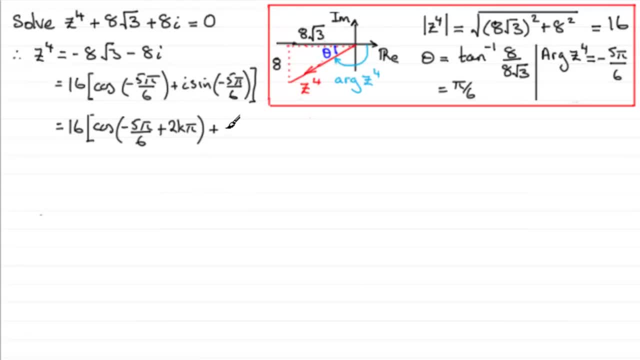 And then we have plus i sine and again minus 5pi over 6 plus 2kpi. And then we have plus i sine and again minus 5pi over 6 plus 2kpi. OK, So that gives us our general result there. 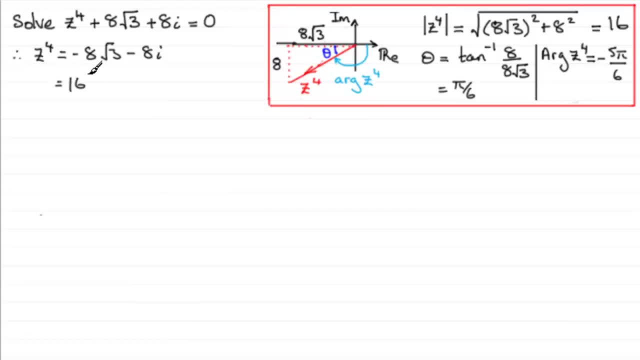 16, and then we can say that this is the same as the cosine of the arg, which is minus 5 pi upon 6, so minus 5 pi upon 6 and then plus i sine of minus 5 pi upon 6.. Now, this is going to have to be written. 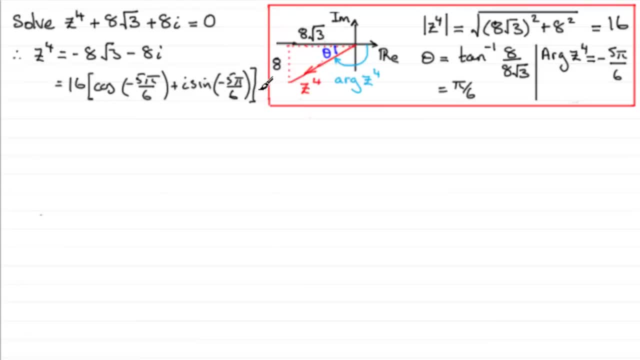 fairly small, because we've got a lot to do in this small space, so I hope you'll understand that that it's going to feel a bit cramped, Okay, well, what we now do, as I've shown you in the cube root circle, is we're going to write z to the power 4 in mod arg form. So I can now rewrite z to the power. 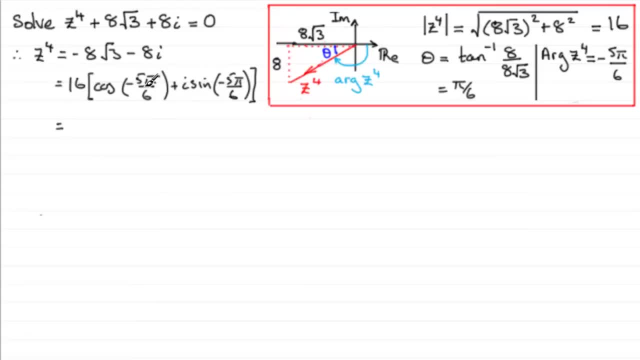 1- if you've seen that video, that we change this arg by adding 2k pi onto each of these angles here, because we can turn in this direction. but if we add any multiple of 2 pi onto this arg, it's always going to take us back to this position, So we'll just change. 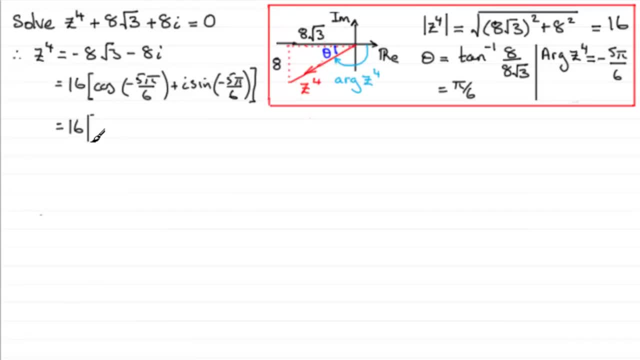 this then to 16, multiplied by the cos of minus 5 pi over 6. but here we add 2k pi. k is an integer, by the way, okay, positive or negative. and then we have plus i sine, and again minus 5 pi over 6, plus 2k pi. 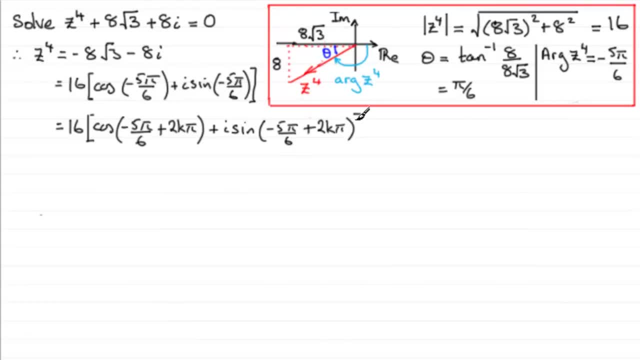 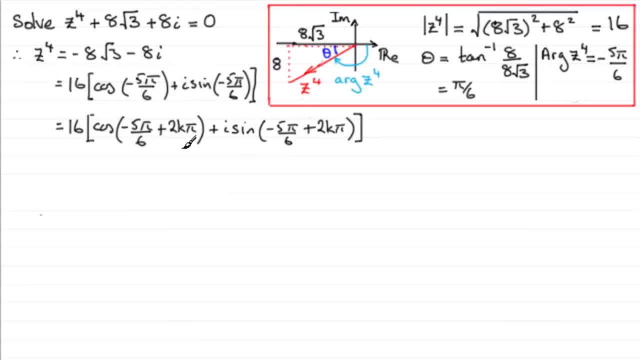 So let's go back to our first example. All right, So this is our first example. Now, to get Z, we need to take the fourth root of all of this. So, because this is made up of two factors, the 16 and the square bracket, it's exactly the same, then, as taking the fourth root of 16.. 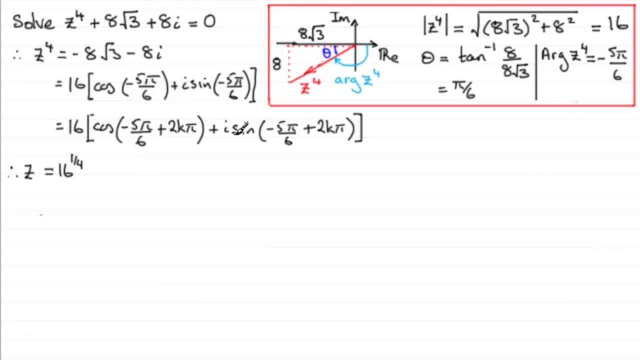 So that would be 16 to the power quarter and the fourth root of this square bracket. To save time, let's just copy that straight in. So that would be 16 to the power quarter. Now, 16 to the power quarter is 2.. Fourth root of 16 is 2.. And now we can use DeMarva's theorem by multiplying each of these angles here by a quarter. 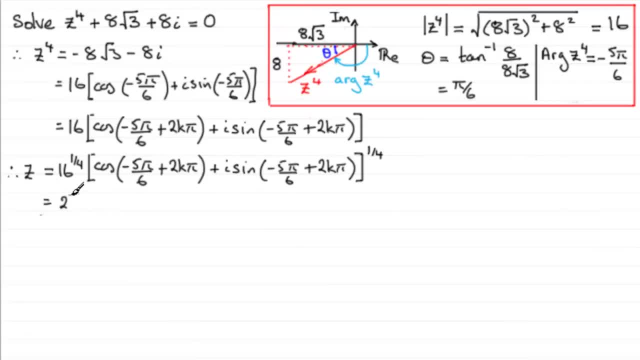 So what we've got then is that for the first one, we've got the cosine of a quarter times minus 5.. So that's going to be minus 5 pi upon 6. That's going to be minus 5 pi on 24.. And then we've got a quarter times 2 k pi, which is going to be k pi on 2.. 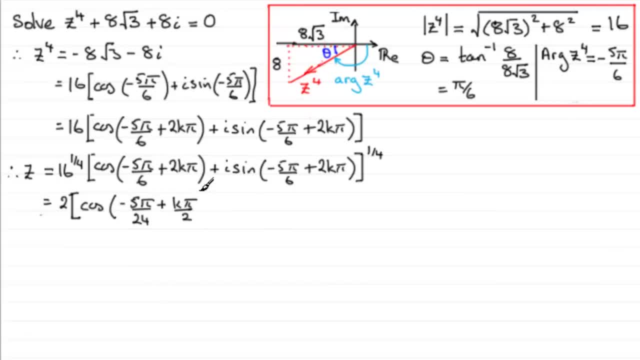 Okay, so k pi upon 2 there, And then we're going to have exactly the same on the sine. So we have again then minus 5 pi on 24.. 24 plus k pi on 2.. Alright, So that's using DeMarva's theorem. 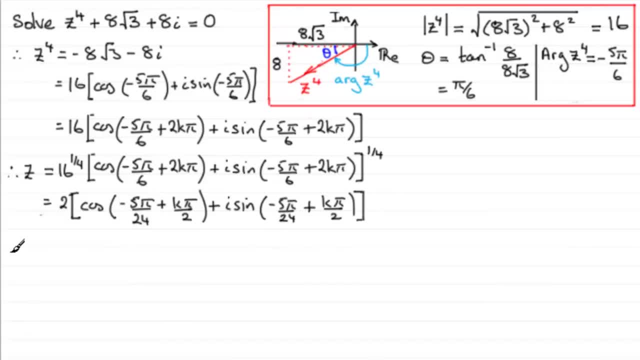 Now, what we need to do now is take integer values for k And we start with when k equals 0. So when k equals 0, z will equal 2.. Okay, we'll just put the 2 down, And then you've got the cosine of. 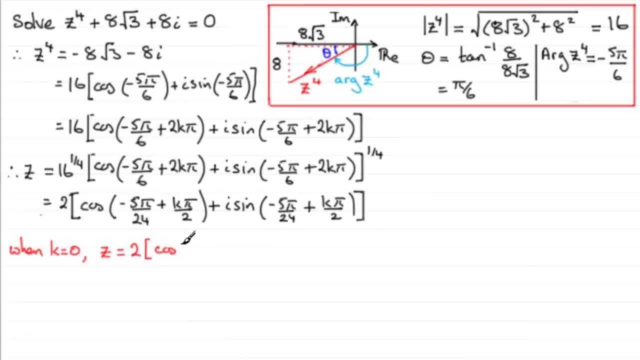 Minus 5 pi over 24.. So we've got minus 5 pi over 24.. And then again the same again with the sine I sine of minus 5 pi over 24.. Okay, so that's one value. Now, next up is when k equals 1.. 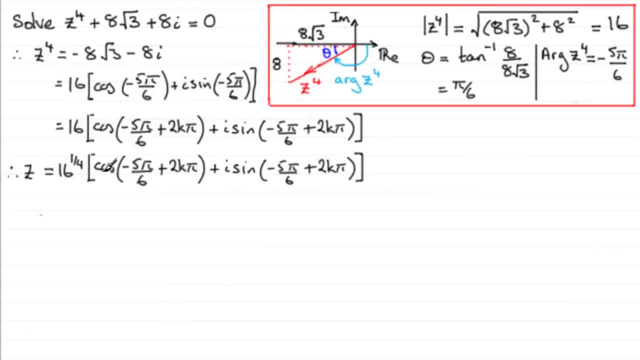 this square bracket. To save time, let's just copy that straight in. okay, so that'd be 16 to the power quarter. Now, 16 to the power quarter is 2, 4th root of 16..2. okay, and now we can use DeMarva's Theorem by multiplying each of these. 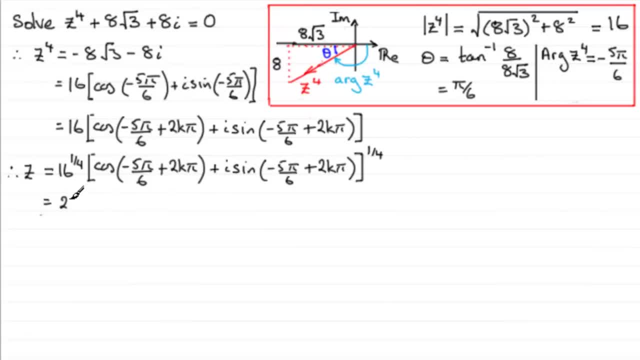 angles here by a quarter. so what we've got then is that for the first one, we've got the cosine of a quarter times minus 5 pi upon 6, that's going to be minus 5 pi on 24, and then we've got a quarter times 2 K pi, which is going to be K pi. 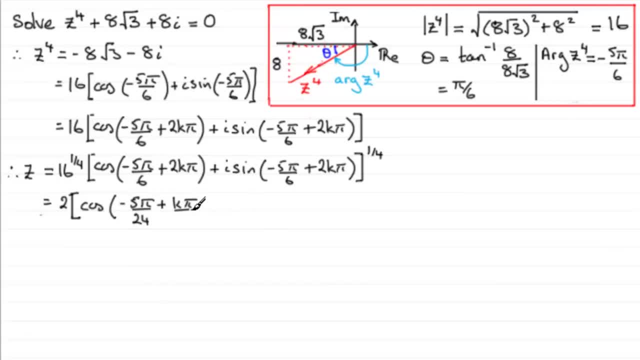 on 2. okay, so K pi upon 2 there, and then we're going to have exactly the same on the sine. so we have again then minus 5 pi on 24, plus K pi on 2. all right, so that's using DeMarva's theorem. now, what we need to do now is take: 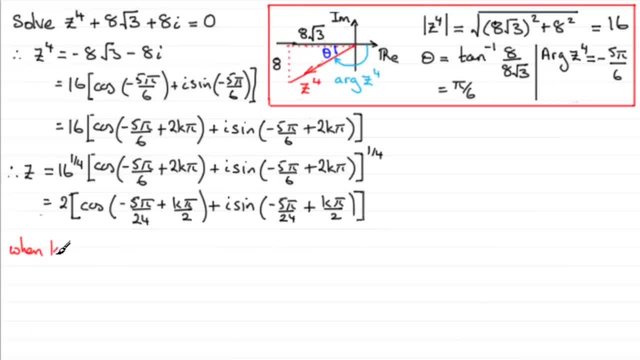 E integer values for K, and we start with when K equals 0. so in K equals 0, Z will equal 2. okay, we'll just put the 2 down, and then you've got the cosine of minus 5 pi over 24. so minus 5 pi over 24, and then again the same again with the sine. 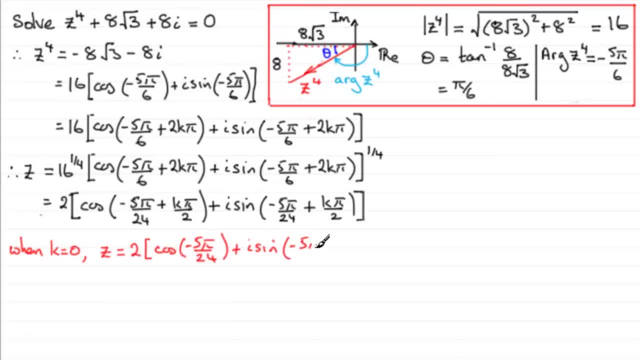 I sine of minus 5 pi over 24. okay, so that's one value. the next up is when K equals 1. when K equals 1, what you've got is that Z again equals 2, but this time the argument will change. when K equals 1, we've got minus 5 pi upon 24, plus pi on 2. 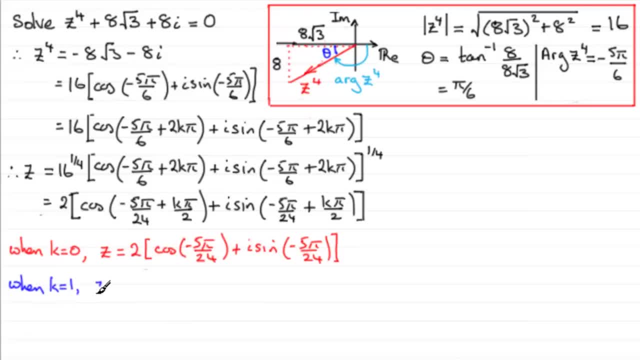 When k equals 1. What you've got is that z again equals 2.. But this time the argument will change. When k equals 1, we've got minus 5 pi upon 24, plus pi over 2. And that comes to 7 pi over 24.. 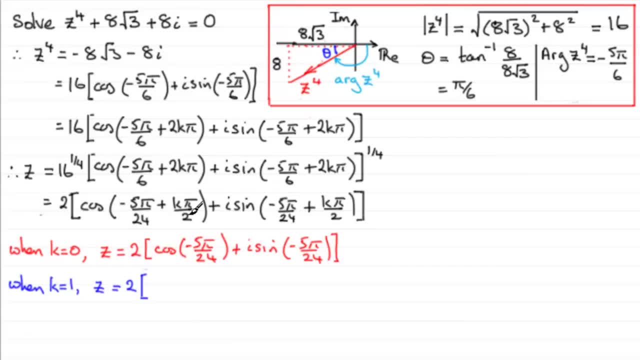 And as an arg for a complex number that's fine because it lies in the range Greater than minus pi radians, but less than or equal to pi. So we would end up with the cosine of 7 pi over 24 plus and again i sine of 7 pi over 24.. 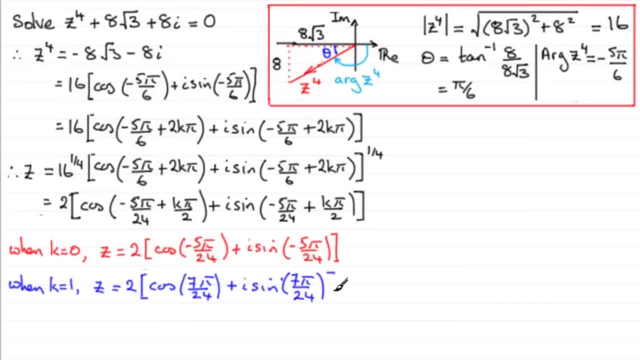 Okay, so that's when k equals 1.. Now when k equals 2.. Let's just put that in: When k equals 2.. What do we get? Well, z equals, again, it will be 2.. And if we substitute 2 into here, we've got 2 pi over 2.. 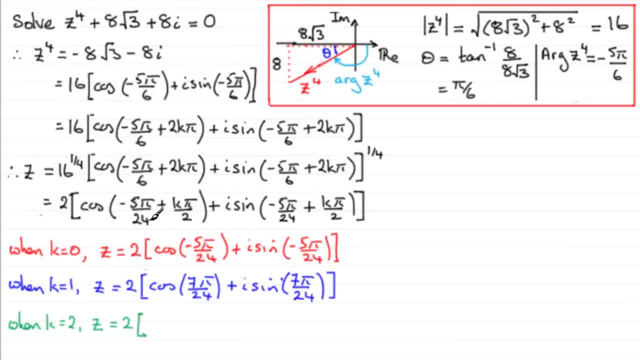 In other words pi radians. And then we subtract 5 pi upon 24.. So again, that's going to be well within our range for the argument between minus pi and less than or equal to pi radians, Because It comes out at 19 pi over 24.. 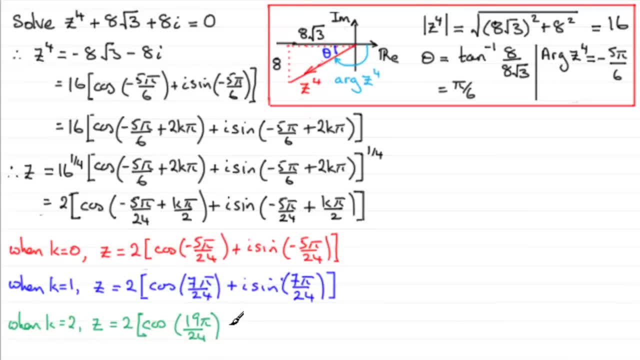 19 pi over 24. then, And then we've got the same for the sine, The i sine, of 19 pi over 24.. Okay, so we now know that we've got 4 solutions. So it seems natural to take k equals to 3.. 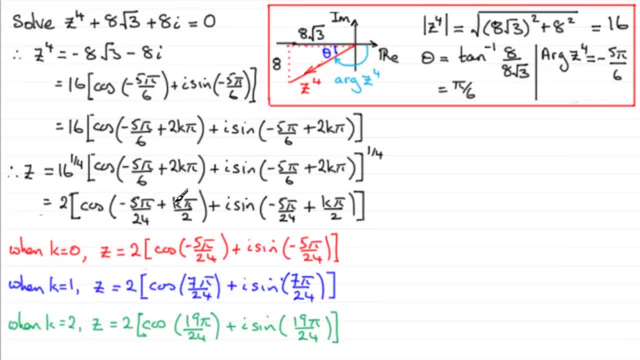 If you take k equal to 3 here, What happens is you end up with 3 pi over 2, minus 5 pi over 24. Which in fact gives you 31 pi over 24. That exceeds pi radians. So what we do is we take k equal to negative 1.. 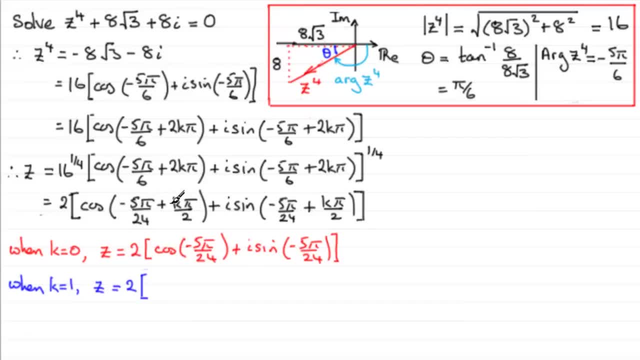 over 2, and that comes to 7 pi over 24, and as an arg for a complex number, that's fine because it lies in the range greater than minus pi radians but less than or equal to pi radians. so we would end up with the cosine of 7 pi over 24 plus- and again i sine- of 7 pi over 24. okay, so that's when. 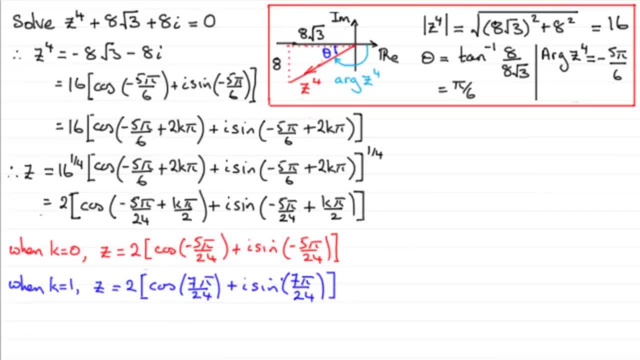 k equals 1. now when k equals 2, let's just put that in: when k equals 2, what do we get? well, z equals again, it will be 2, and if we substitute 2 into here, we've got 2 pi over 2. 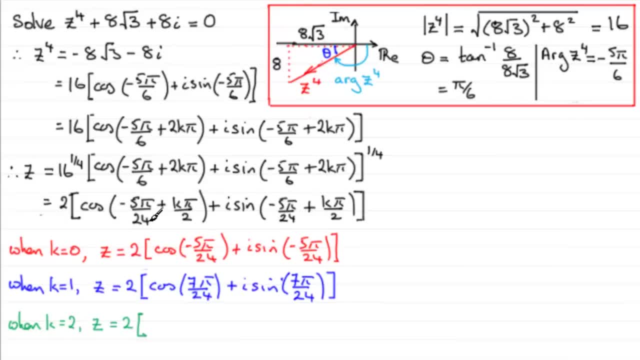 in other words pi radians, and then we subtract 5 pi upon 24, so again that's going to be well within our range for the argument between minus pi and less than or equal to pi radians, because it comes out at 19 pi over 24. 19 pi over 24 then, and then we've got the same for the sine, this i sine- of 19 pi over. 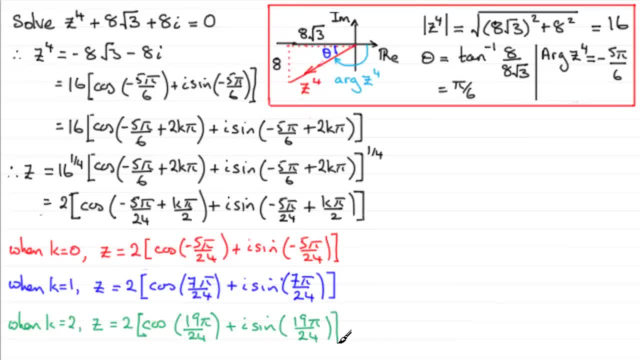 24. okay, so we now know that we've got four solutions. so it seems natural to take k equals to 3. if you take k equal to 3 here, what happens is you end up with 3 pi over 2 minus 5 pi over 24, which in fact gives you 31 pi over. 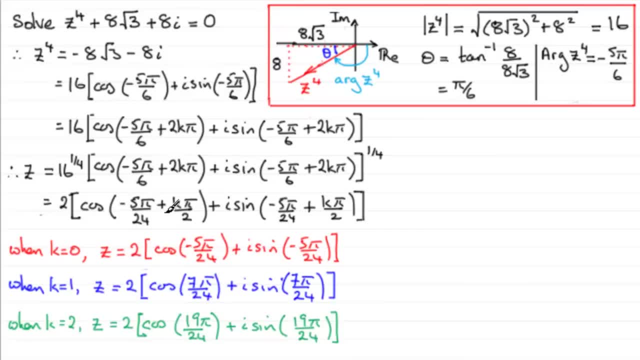 24 that exceeds pi radians. so what we do is we take k equal to negative 1 and when k equals negative 1, that gives us an angle in range. okay, when k is negative 1, you get minus pi over 2, minus 5 pi over 24 and that comes out to minus 17 pi over 24 radians. so if we write this: 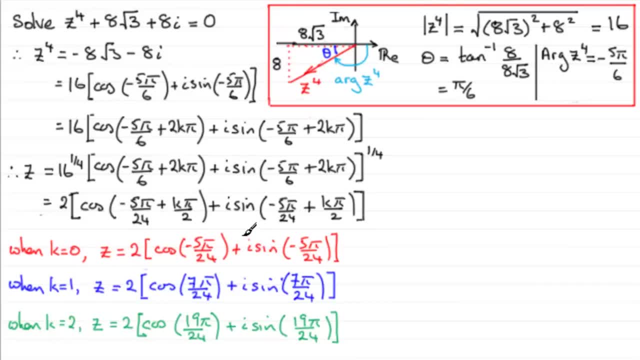 And when k equals negative 1, that gives us an angle in range. Okay, When k is negative 1, you get minus pi over 2, minus 5 pi over 24. And that comes out to minus 17 pi over 24 radians. 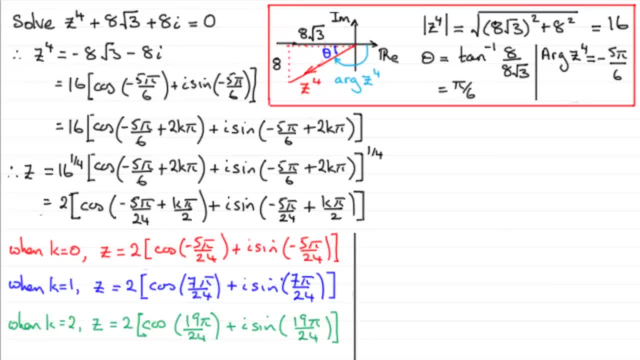 So if we write this down here, what we've got is that when k equals minus 1, z equals 2 times the cosine of minus 17 pi over 24.. And then plus i sine of Minus 17 pi over 24.. 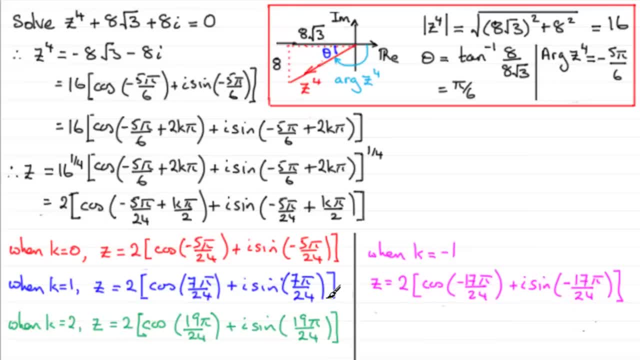 Now we didn't have to write our answers in mod? r form. What we could have done is written them in exponential form, And if that were the case, then these would have been our answers. We could have said: or z equals 2e to the i theta, where theta equals minus 5 pi over 24.. 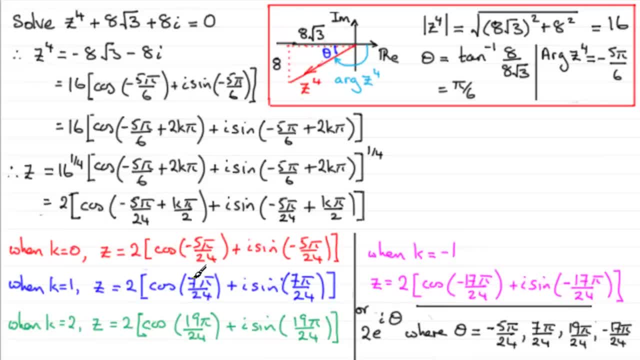 We had here 7 pi over 24.. Or 19 pi over 24.. Or minus 17 pi over 24.. Now an interesting result always occurs when you're doing questions like this, When you're trying to find the nth roots of a particular value. 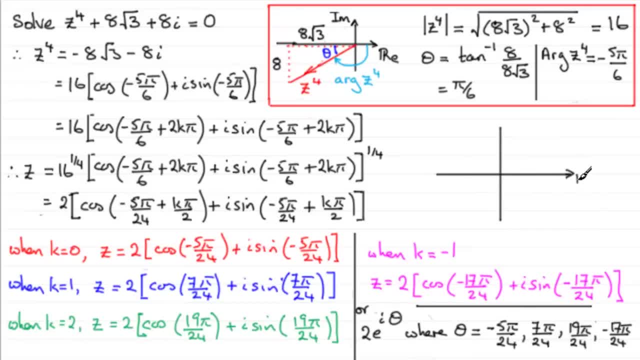 Because if we look at the argon diagram, Let's just draw our real axis and our imaginary axis. What happens Is that our roots have always got the same modulus- Okay, 2 in this particular case. So, in other words, they are all going to lie on a circle of radius 2 units. 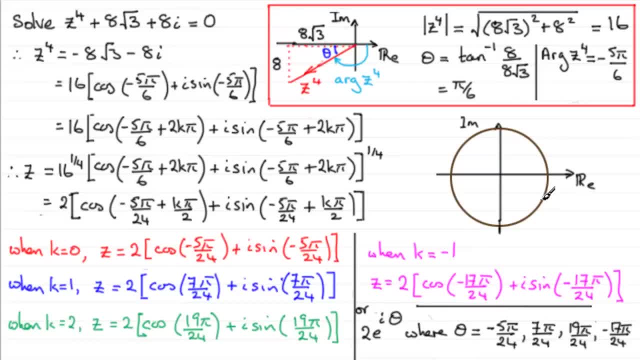 Now, if we just extend that a little bit, If we take the first result when k was 0. You can see that we've got a complex number, a root with an argon. It's going to be minus 5 pi over 24.. 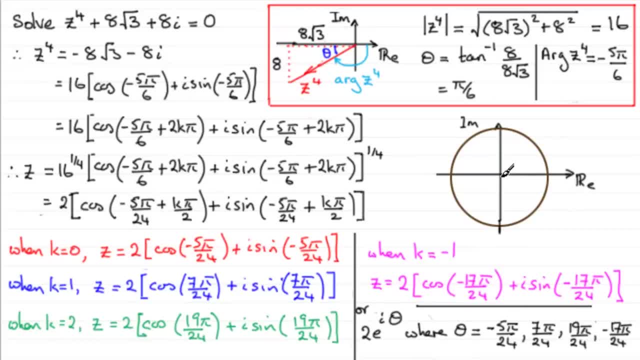 So if we were to draw that in- okay, it's going to look something- say like this: Okay, So that is z1, if you like, Let's just mark that in as z1.. Put that as z1.. 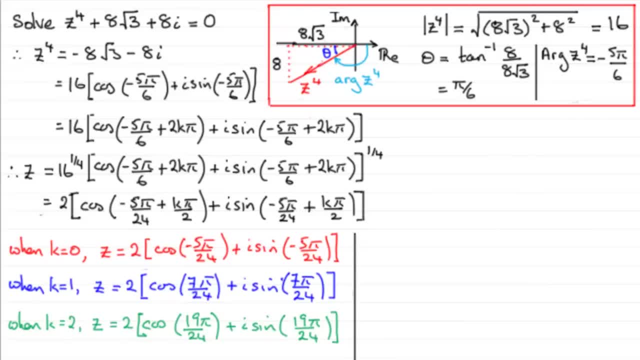 down here. what we've got is that when k equals minus 1, z equals 2 times the cosine of minus one. z equals 2, 17 pi over 24, and then plus i sine of minus 17 pi over 24. now we didn't have 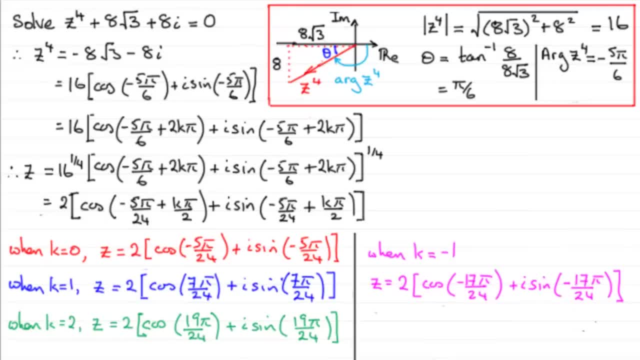 to write our answers in mod art form. what we could have done is written them in exponential form, and if that were the case, then these would have been our answers. we could have said: or Z equals 2e to the i theta, where theta equals minus 5 pi over 24. we had here 7 pi over 24, or 19 pi over 24, or minus 17 pi over. 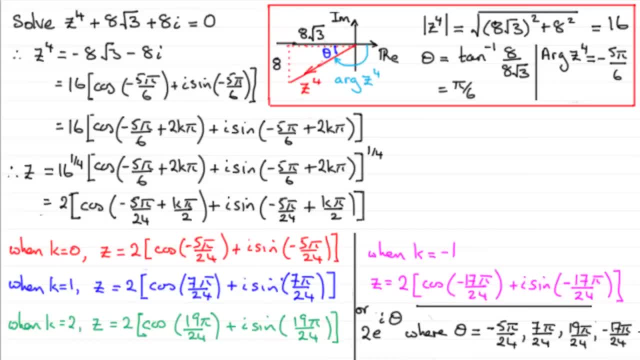 24. now, an interesting result always occurs when you're doing questions like this, when you're trying to find the nth roots of a particular value, because if we look at the argon diagram, let's just draw our real axis and our imaginary axis. what happens is that our roots have always got the same. 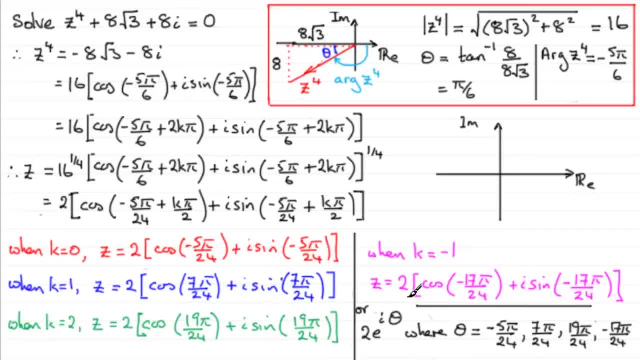 modulus, okay, two in this particular case. so in other words, they are all going to lie on a circle of radius two units. now if we just extend that a little bit, if we take the first result when K was zero, you can see that we've got a. 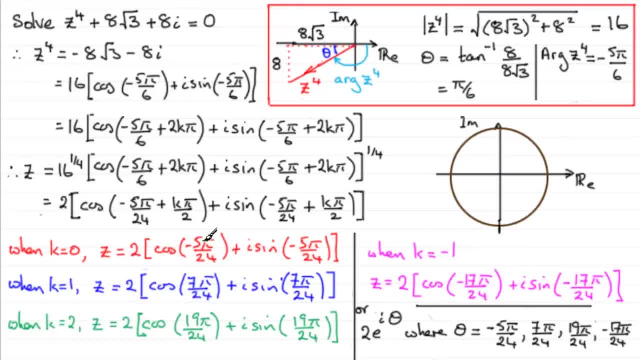 complex number, a root with an argon minus 5 pi over 24. so if we were to draw that in: okay, it's going to look something say like this: okay, so that is Z 1. if you like, let's just mark that in as Z 1. put that as Z 1. 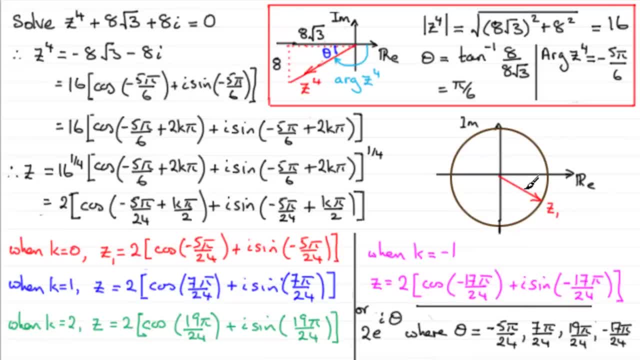 this angle here then being minus 5 pi upon 24 radians, its magnitude obviously is 5 pi upon 24, but returning in a clockwise sense. so therefore minus 5 pi upon 24 when K equals 1. if we were to plot this on the argon diagram, what we 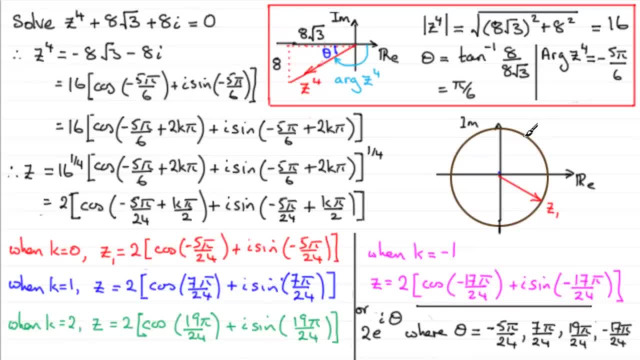 would find is that it is a complex number up here. say that this then is Z2.. Mark that in as Z2.. This angle in here is 7 pi upon 24.. Now, if you add it to the 5 pi upon 24 here, what you find is that you get pi upon 2, the equivalent of a right angle. 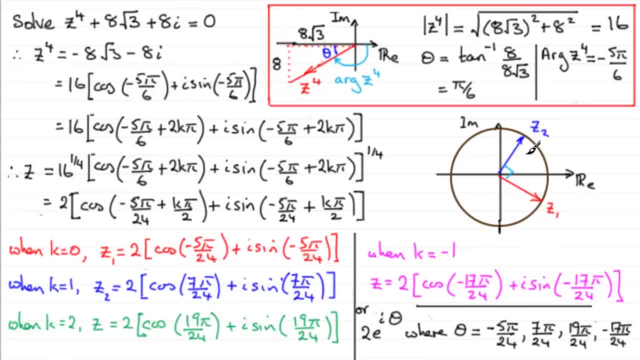 And this happens. You'll find that we've got four roots in this example: Z1, Z2, Z3, and finally Z4. And all these four roots are equally spaced around the argon diagram. Okay, if we were to draw. 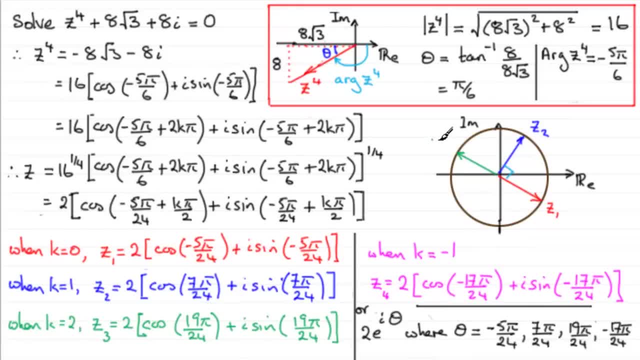 Z3 in, okay, it would be out here. Z3, and finally Z4.. Z4 would be down here, Okay. so hence the colour coding that I did. Each of these angles in here is a right angle, pi upon 2 radians. So you could argue that once you've got one particular root. 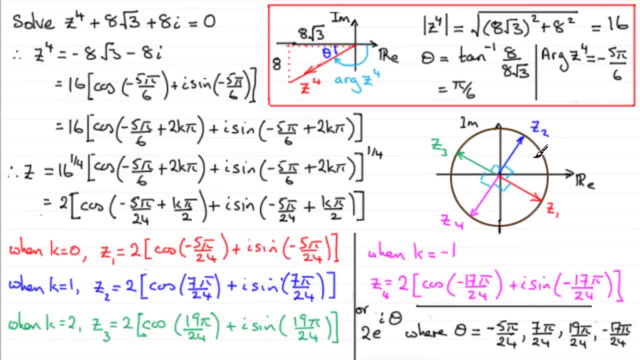 you could divide 2 pi up into n divisions- Okay, whatever your nth, how many roots you're doing? And then you could just simply step them off round the circle. So I hope you can use this example to use as a basis for doing similar. 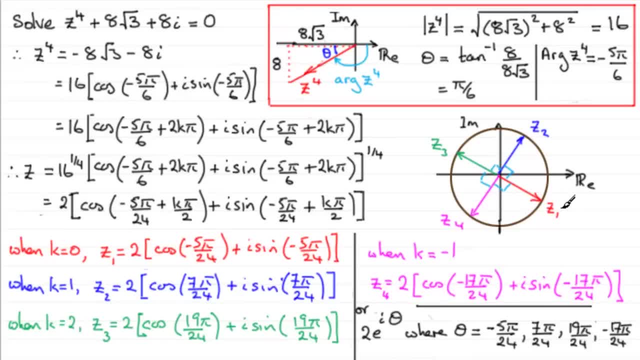 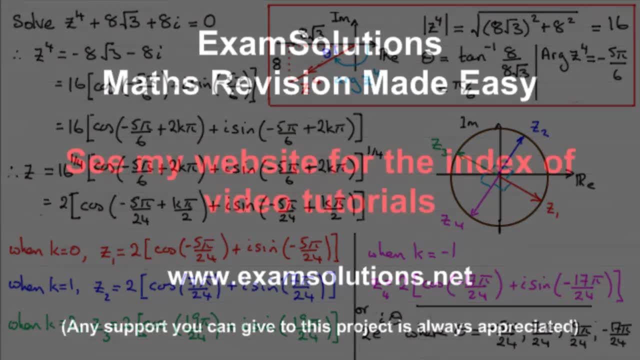 examples where we apply DeMarva's theorem. Okay Subtitles by the Amaraorg community. 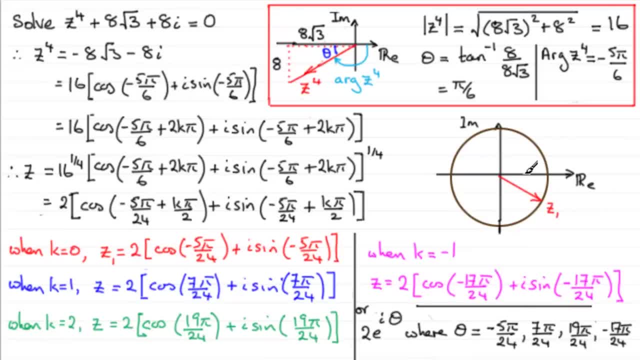 This angle here then being minus 5 pi upon 24 radians, Its magnitude obviously is 5 pi upon 24 radians, So it's going to be minus 5 pi upon 24, but returning in a clockwise sense, So therefore minus 5 pi upon 24.. 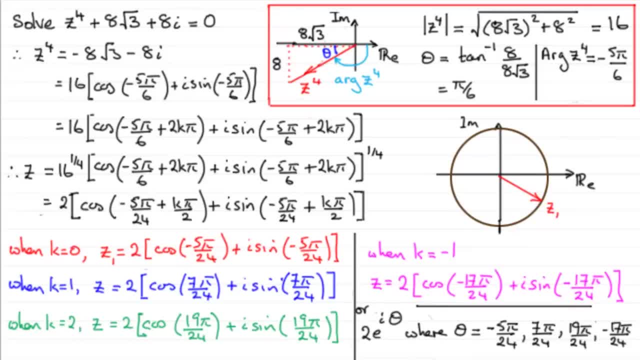 When k equals 1, if we were to plot this on the argon diagram, what we would find is that it is a complex number up here. Let's say that this then is z2.. Mark that in as z2.. This angle in here is z1.. 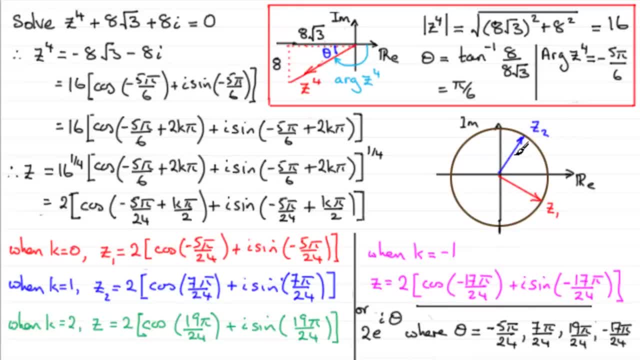 This angle in here is z2.. This angle in here is z1.. This angle in here is z2.. This angle in here is z1.. This angle in here is z2.. This angle in here is 7 pi upon 24.. 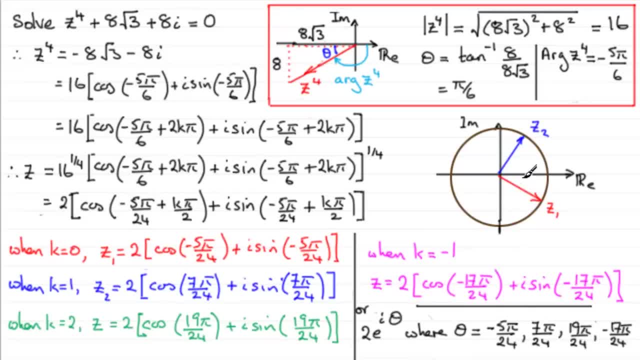 Now, if you add it to the 5 pi upon 24 here, what you find is that you get pi upon 2, the equivalent of a right angle, And this happens. You'll find that we've got four roots in this example: z1, z2, z3,. 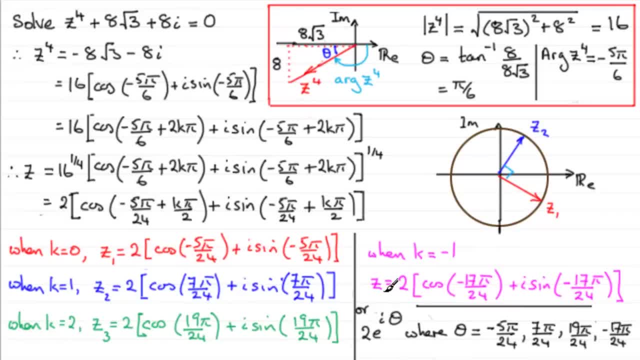 and finally, z4. And all these four roots are equally spaced around the argon diagram. OK, If we were to draw z3 in, OK, it would be out here z3. And finally, z4 would be down here, OK. 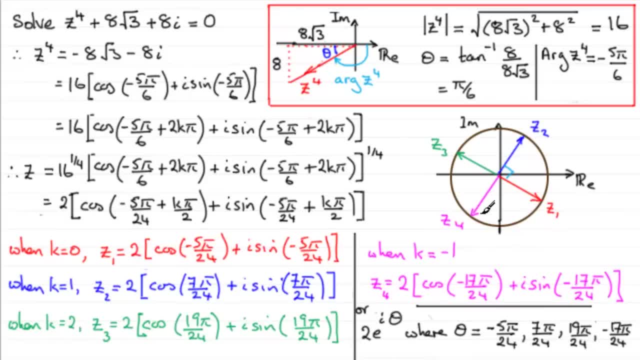 So hence the color coding that I did. Each of these angles in here is a right angle, pi upon 2, radians. So you could argue that once you've got one particular root, you could divide 2 pi up into n divisions. OK, 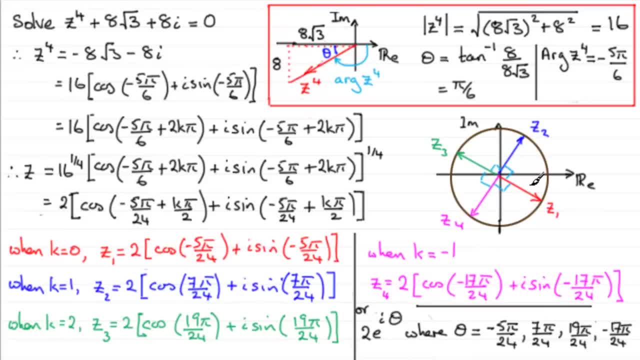 whatever your nth, how many roots you're doing, And then you could just simply step them off round the circle. So I hope you can use this example to use as a basis for doing similar examples where we apply DeMarva's theorem. OK,